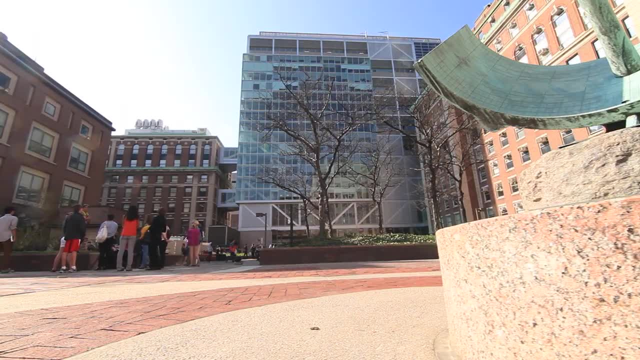 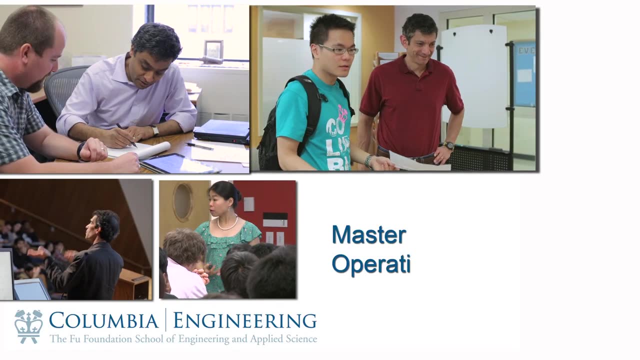 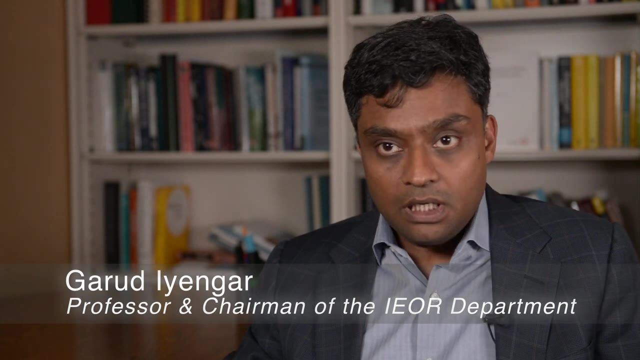 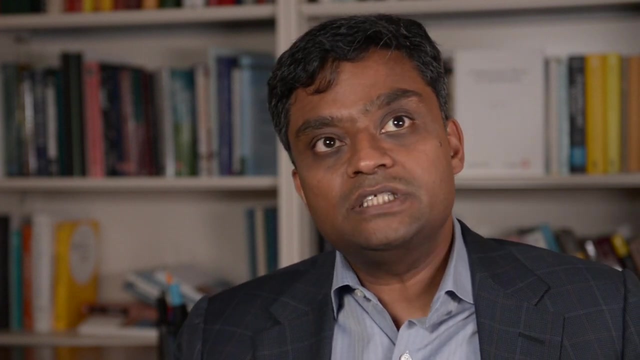 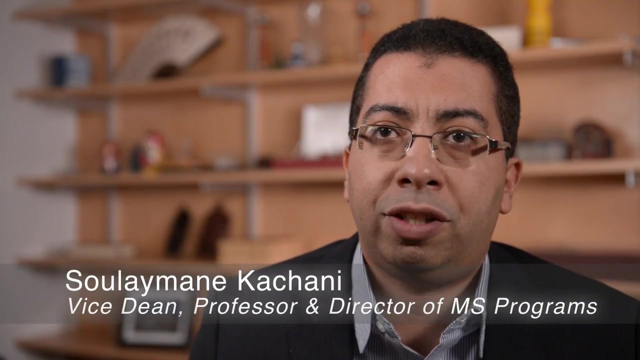 The MS-OR program starts off with a core in optimization, deterministic models, stochastic models, simulation, probability and statistics, which forms the core that will then be taken and refined through electives in different areas. The MS program in operations research has five concentration areas: Financial and managerial. 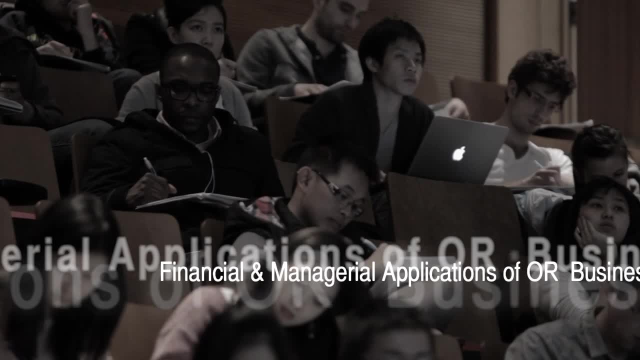 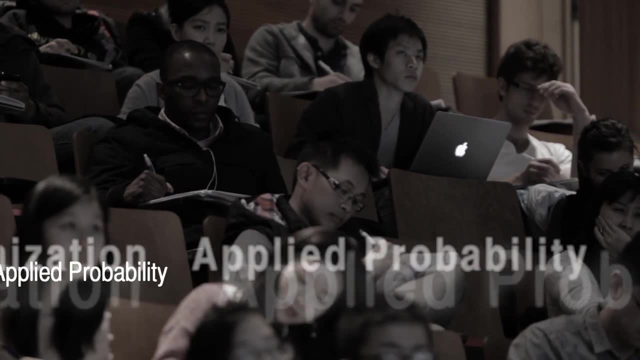 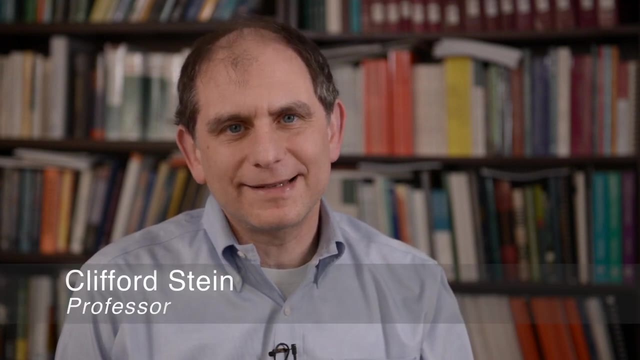 applications of OR, business analytics, logistics and supply chain management, as well as two concentration areas in optimization and applied probability. Many people ask what operations research is. My definition is that it's applying the techniques and methodologies of science and engineering to nontraditional engineering problems. It's 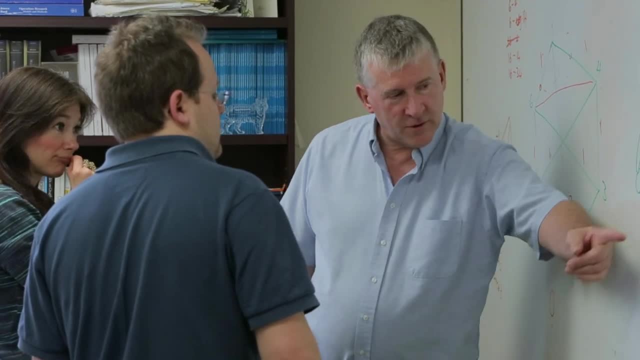 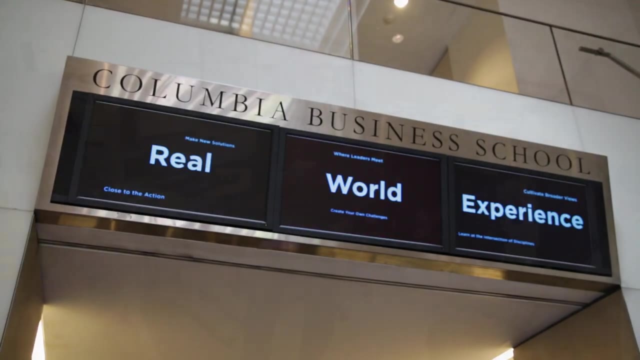 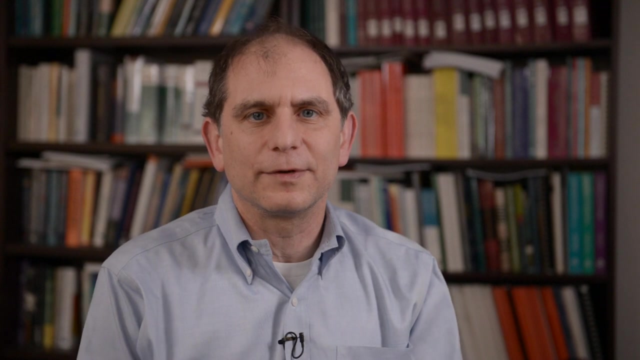 inherently very multidisciplinary and that leads us to different areas and also to collaborations with people in other departments at Columbia, such as the business school, the computer science department, the electrical engineering department, earth and environmental studies, civil engineering. So we look widely for different problems and it's really the role of someone. 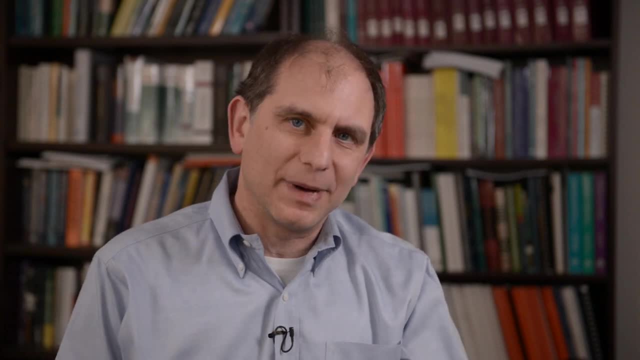 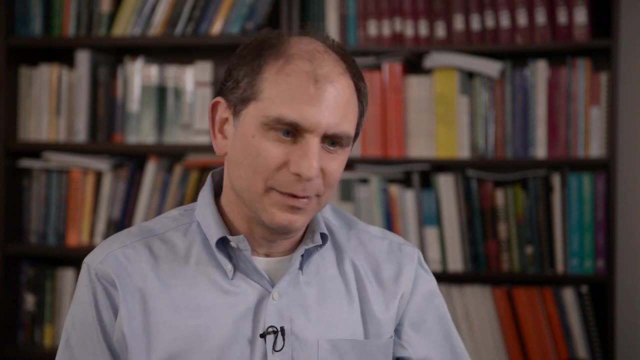 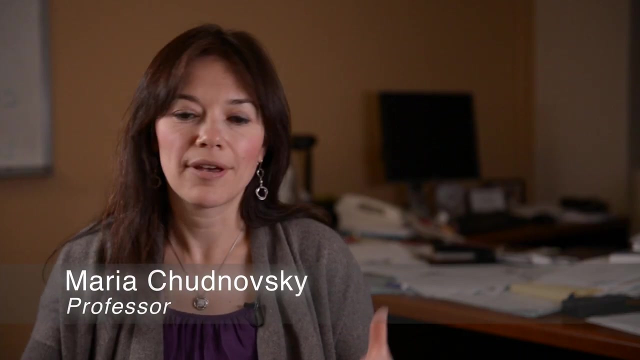 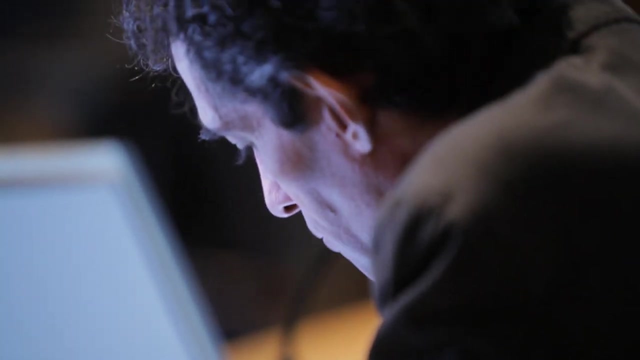 in operations, research, to take those problems and model them and turn them into a mathematical problem that we can then use our solution method. This is a very strong department. A lot of people are doing some sorts of mathematics. basically, One of the big areas that we use a lot is probability theory, by which I mean randomness. 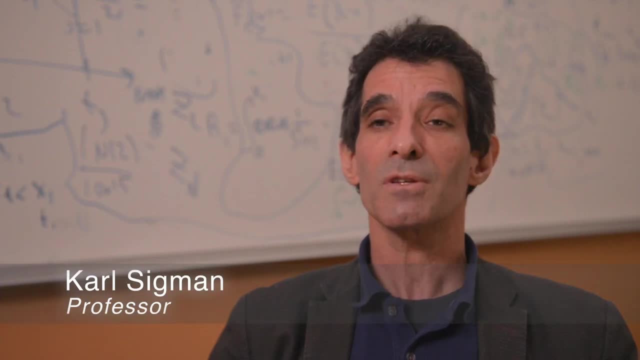 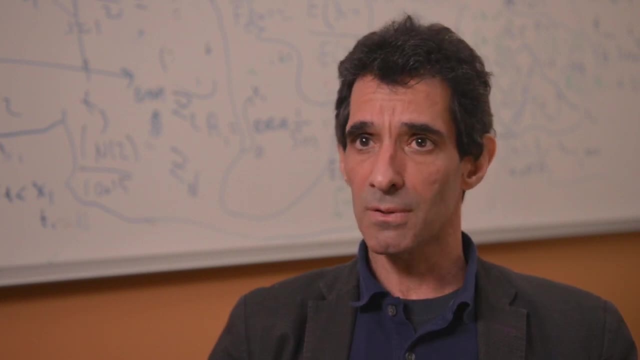 The computer can actually hand you numbers as if they're truly random. A computer can flip coins for you, And if a computer can flip coins for you, it can build models for you, And that's what's the key to using probability theory. 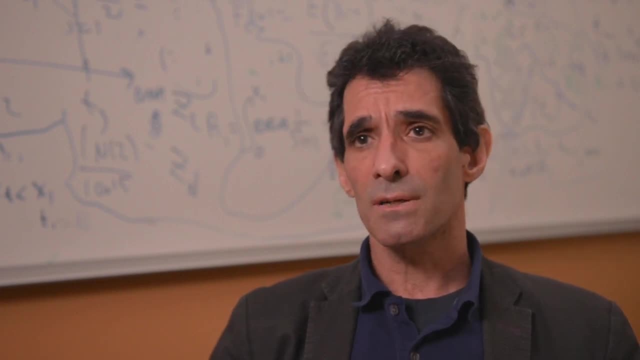 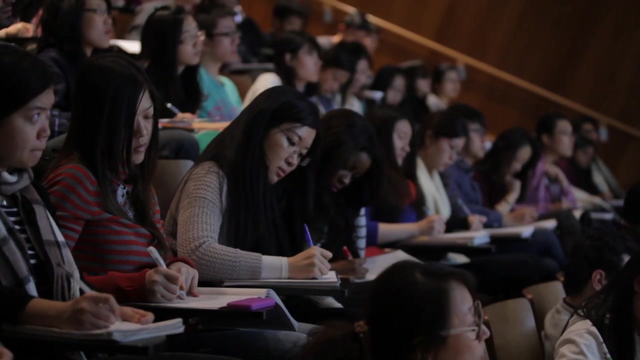 The other part the department would be strong in is this optimization part, which pretty much means, once you have a problem specified, how do you then solve, how to find the best thing to make it work? Students always learn the basics of that kind of methodology too. 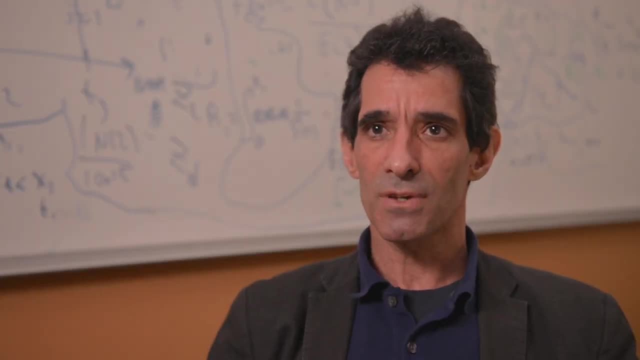 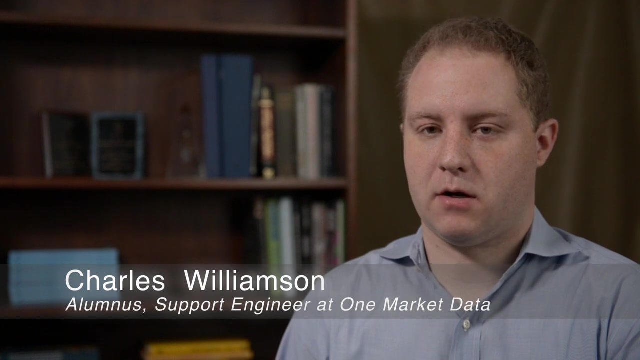 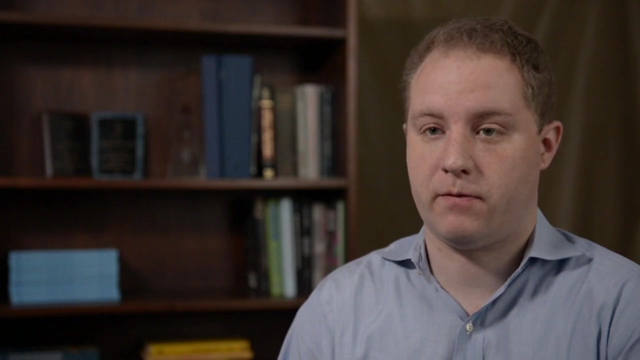 Those are the two traditionally main OR fields, which is optimization and we call it stochastic modeling. One of the things that an OR degree helps me with is that Columbia is very strong in teachingate stochastic processes and the underlying math behind most of the theory, behind financial